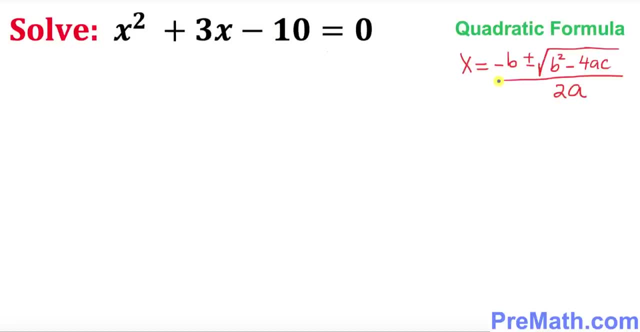 formula. So here is the quadratic formula and we're going to be solving this quadratic equation. Let's go ahead and find out what are our coefficients. Right here, the leading coefficient a is 1 by default, So a equals to 1.. Our b coefficient, b, is positive 3 and c is simply. 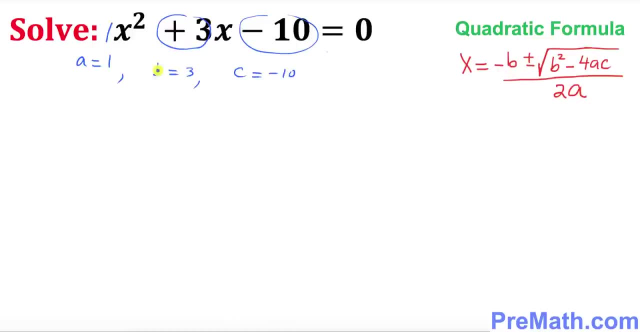 negative 10.. Let's go ahead and solve this given quadratic equation by quadratic formula. Then plug it in in this formula. So this is pretty much going to become x equal to minus. b means negative. b is 3 plus or minus b square is 3, square minus 4 times a is 1 and c is negative. 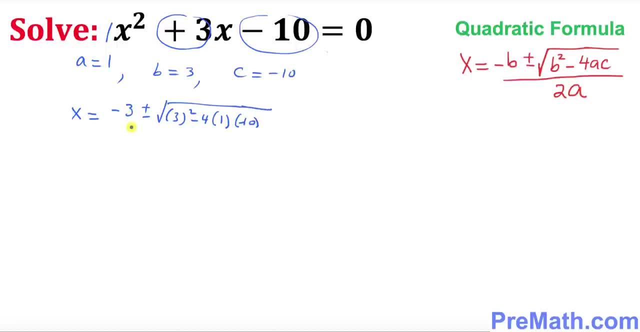 10. Isn't it Divided by 2 times 1.. Now let's go ahead and simply simplify it. Negative 3 plus minus 3 square is 9.. See this negative and negative become positive: 40 divided by 2 times 1 is 2.. So that's going to give us negative 3 plus or. 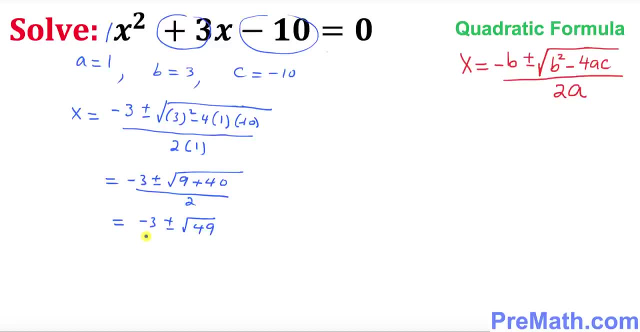 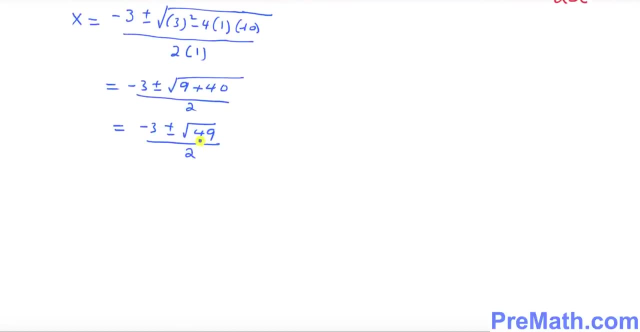 minus, This becomes 49 divided by 2.. Now you know that 49 is a perfect square, So let's go ahead and simplify it. Negative, 3 plus minus, square root of 49 is 7 divided by 2.. Now we're going to go ahead and split these signs: Once it's positive and then negative. 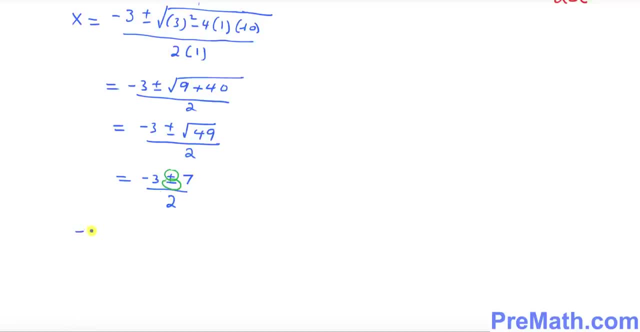 So that's pretty much- is going to give us negative 3 plus 7 divided by 2.. And the other is going to become negative 3 plus minus. square root of 49 is 7 divided by 2.. So that's going to. 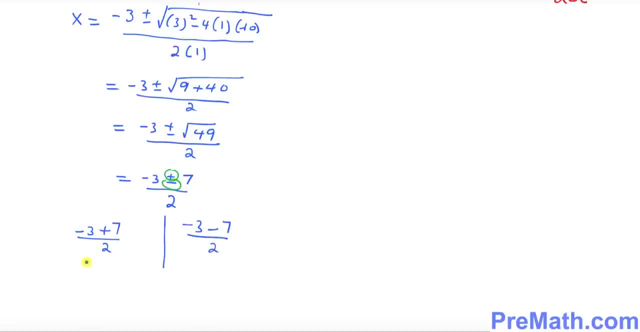 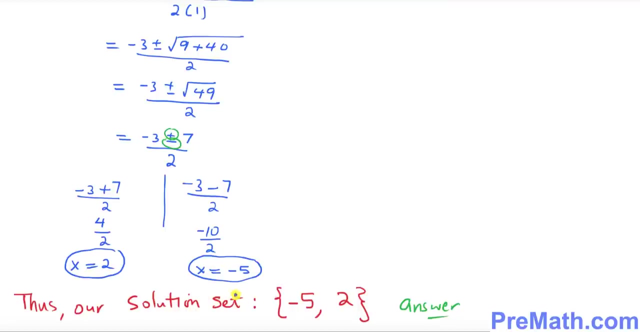 give us 4 over 2 means x is going to be. our solution is 2.. So let's go ahead and do on this side. That's going to become negative 10 divided by 2.. So x is going to be equal to negative 5.. So these are our two solutions. Thus our solution set turns out to be a negative. 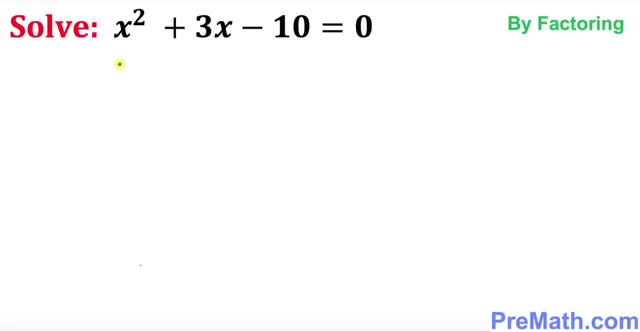 5 and 2.. Now we're going to solve this quadratic equation by factoring technique. So how are we going to do the factors? Just simply put two parentheses And set it equal to 0.. What are the possible factors? One of them is going to be x minus 2.. 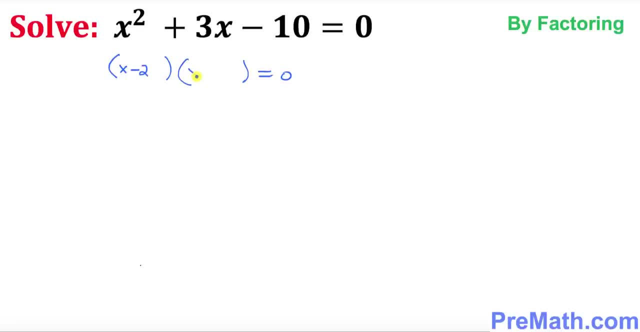 And the other one is going to be x plus 5.. All right, So now, how do you know that thing? These numbers negative 2 and positive 5, if you multiply them, that's going to give you this last number, negative 10.. 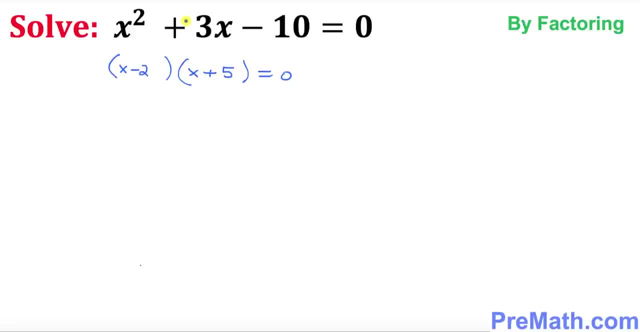 And if you add these two numbers, that is going to give you positive 3, the middle number. So the next step is I want you to go ahead and split them up, So x minus 2 equal to 0.. And the other? 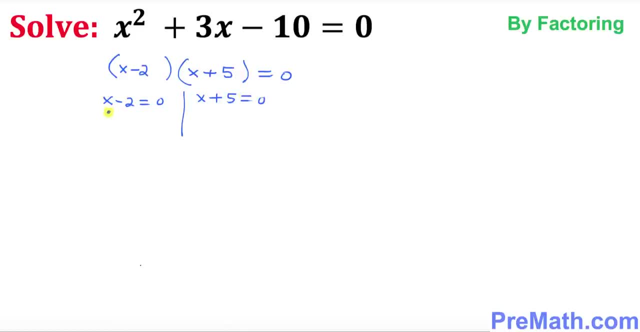 one is x plus 5 equal to 0. So that means x equal to positive 2 is one of the solution And x equal to negative 5 is another solution. Thus our solution set Set turns out to be a negative 5 and 2.. And finally, we're going to solve this quadratic equation by: 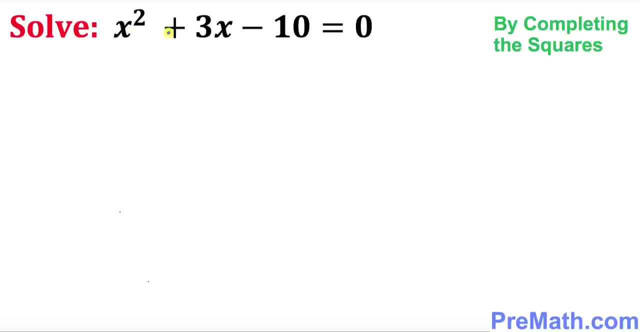 completing the square, The very first step. what I want you to do is go ahead and leave only x's on the left hand side, And the rest of stuff should be on the other side. That means I want to add 10 on both. 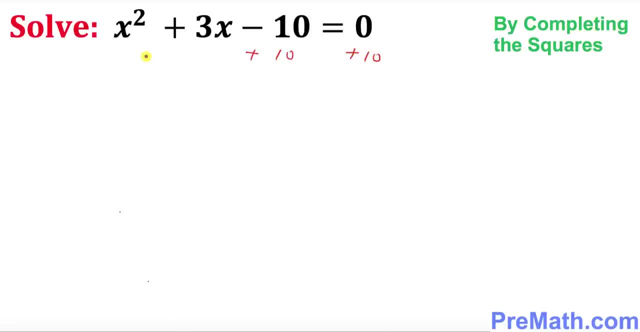 sides to make sure that 10 goes on the other side. So once you do that one, So that's going to simply this cancels out. so we got x squared plus 3x equals to positive 10.. So the next step, what we're going to do, is I want you to just focus on the coefficient of x, the middle part over here, this one over here 3.. 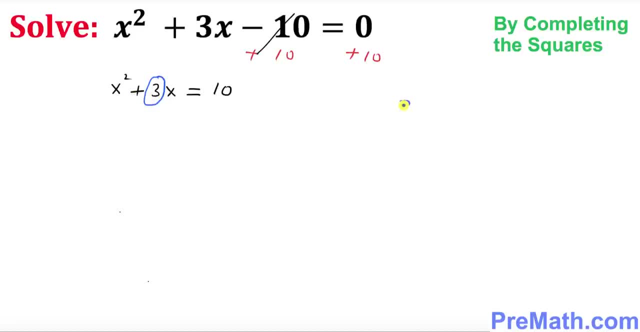 Don't worry about this sign, just 3.. I want you to write it right up here, and then I want you to divide it always by 2, and then, finally, I want you to square it. So, whatever this quantity, I got this thing. we're going to go ahead and add on both sides of this equation. 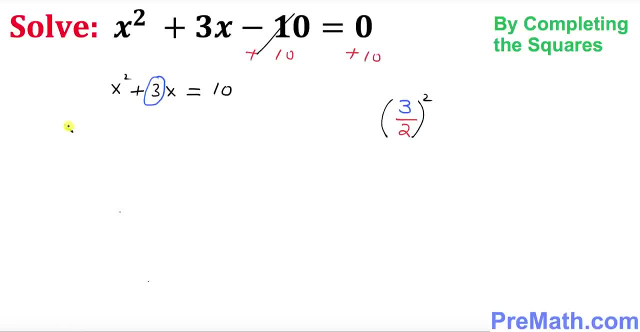 So that means this is the way I'm going to do: x squared plus 3x plus and on this side, 10 plus. okay, So now, whatever this quantity I got, I'm going to just go ahead and add on both sides. 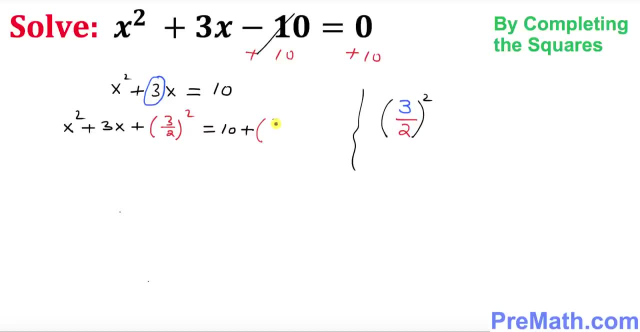 3 over 2 squared on this side and 3 over 2 squared Now. I want you to just focus on this side, this part. This is a complete square of x and 3 plus 3 over 2 squared. 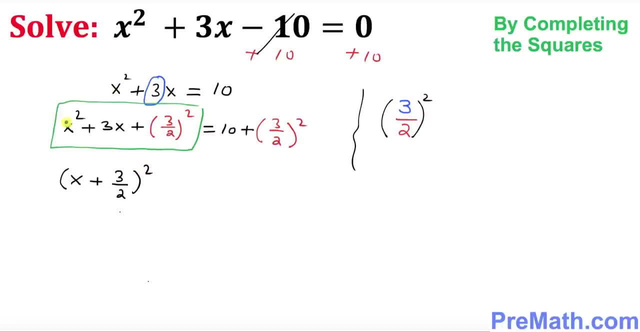 Now you might be wondering: how did I get that one? So this x came over here, This 3 over 2 just simply came over here. And this sign, whatever this sign is, this is just going to come in the middle. 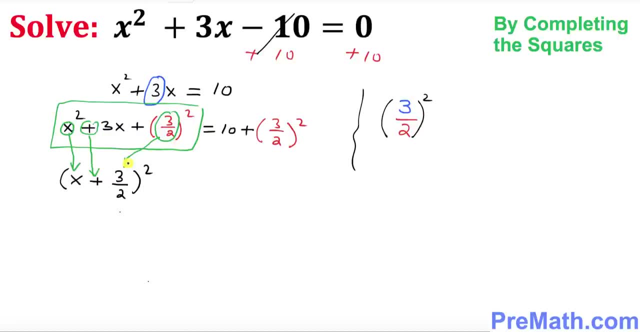 So always, this is the rule Equals to, so that's going to become 10.. Plus, this 3 over 2 squared becomes 9 over 4.. Now let's go ahead. Let me show you how to add these two numbers. 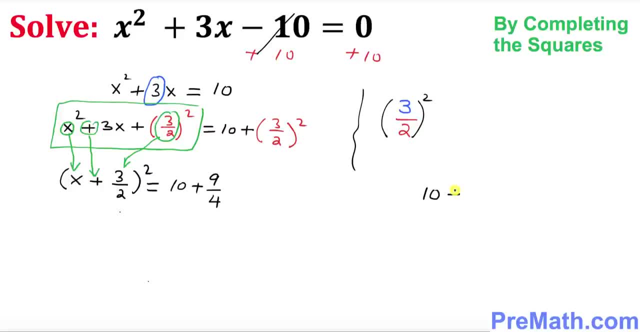 I want you to put down 10,, which is a whole number, plus 9 over 4 is a fraction. When you have a whole number and fraction, you can merge them as a mixed number. This becomes 10 and 9. fourths, 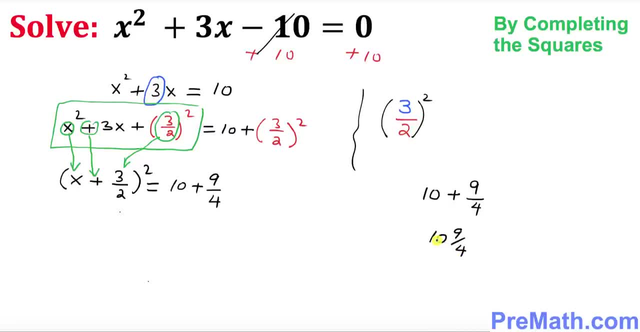 And then you know how to put it in a fraction: 4 times 10 is 40 plus 9.. 49 over 4.. So this becomes 49 over 4 on this side, And this is x plus 3 over 2 squared. 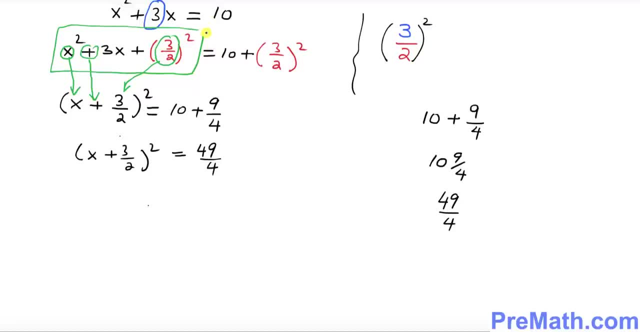 The next. what we want to do is: we want to solve for x, For that one. we need to get rid of this square. We don't want to do square, We want to get rid of this square root on both sides. So this square and square root, they undo each other.